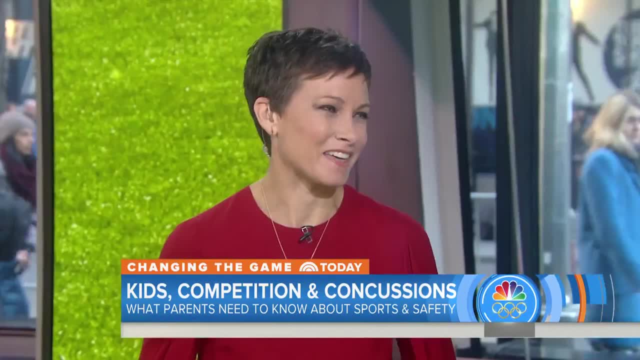 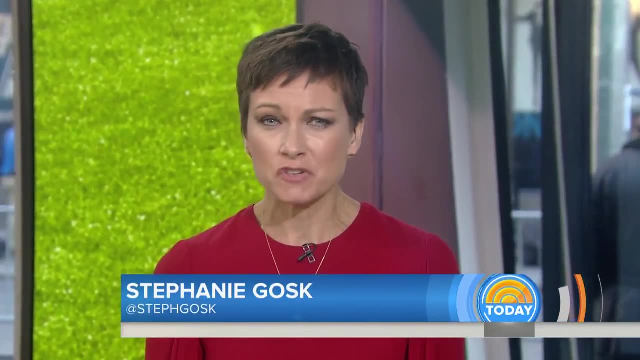 morning with a bit of a different story. Hi again, Hi, thanks, guys. This is an important one. You know, head injuries have been front and center in the conversation about youth sports for years, with parents often sorting through conflicting information or not enough information at all. 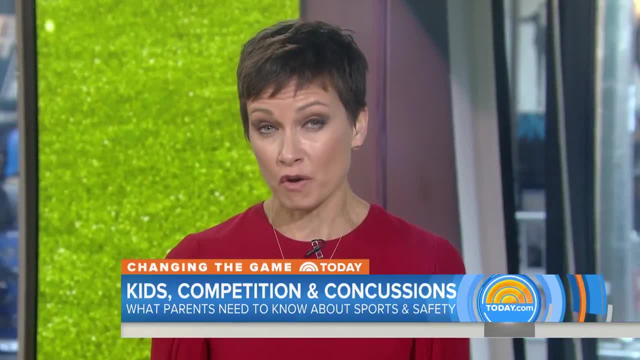 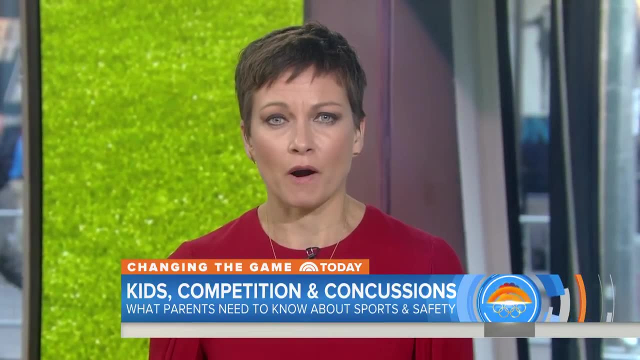 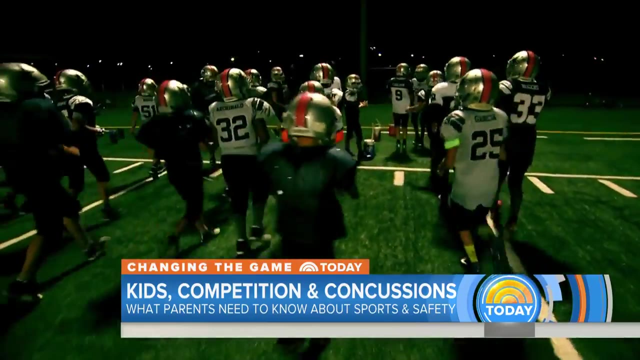 We spoke with coaches, doctors and parents and discovered that, although we are doing better to protect our children's heads, awareness is not where it should be, and many experts say we need to do more. A Tuesday night, just outside of Chicago, the Addison Cowboys practice under the 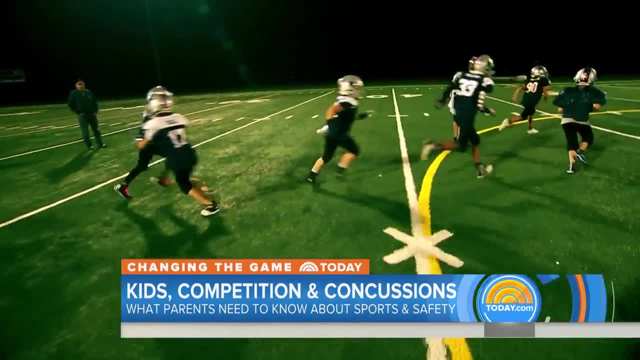 lights. The youth league, with players starting as young as five years old, has been a big part of the conversation. The youth league has been a big part of the conversation. The youth league with players starting as young as five years old has been a big part of the conversation. 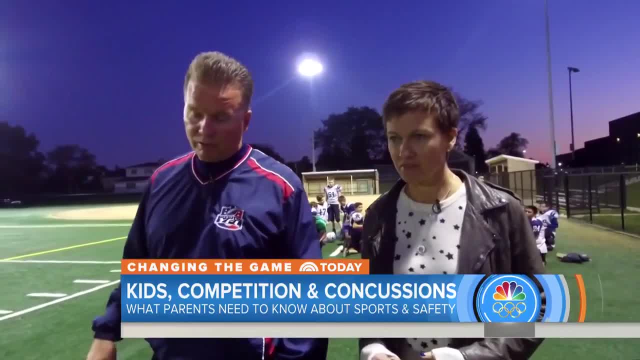 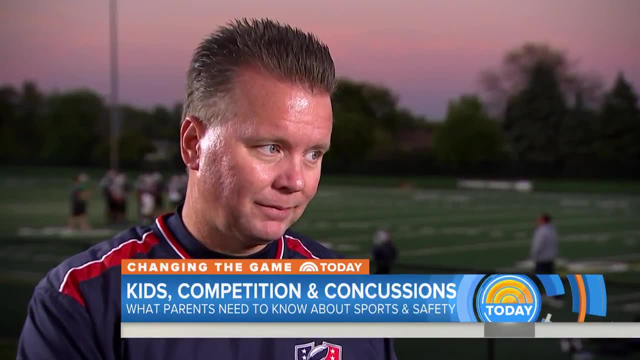 has been around for 60 years. Ron Maxwell has coached for 20 of them. Five six years ago we had 12 teams, so it was 266 kids in the helmet zone And tonight We have 98.. That's it. It's a huge drop. 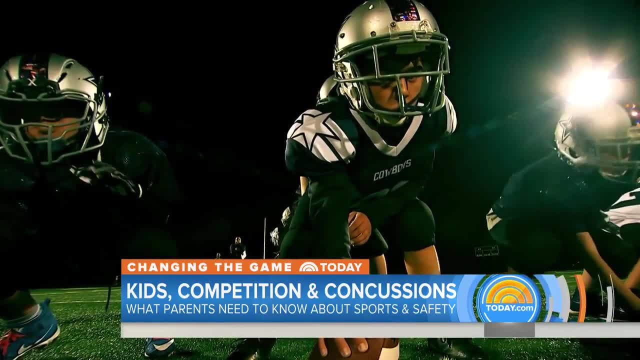 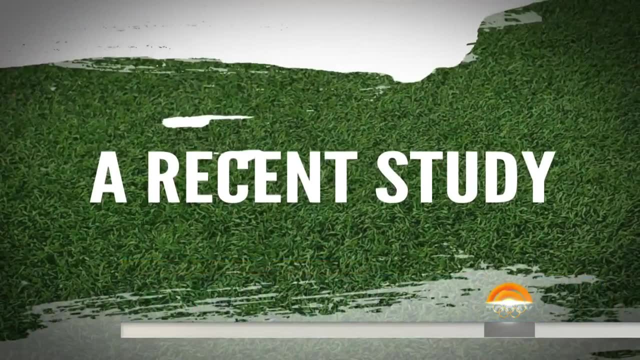 It's a huge drop. Parents are worried about head injuries, which is why the Addison Cowboys have changed their hard-hitting practices. We hit occasionally, but we don't hit too often. A recent study estimated that as many as 2 million sports related concussions are suffered by children under 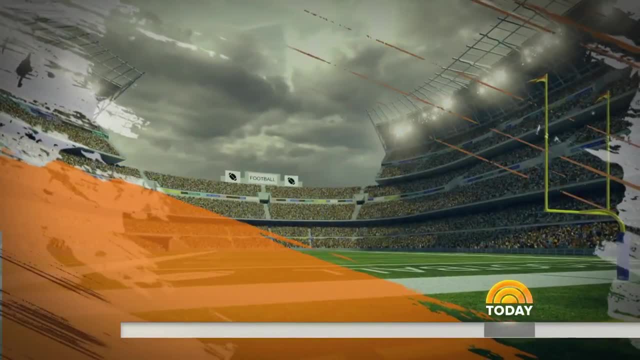 the age of 18.. The Addison Cowboys have been a big part of the conversation. The Addison Cowboys have been around more than 2000 sports related. the teams and coaches have been doing a good job not only at this point but at all at the end of the year. 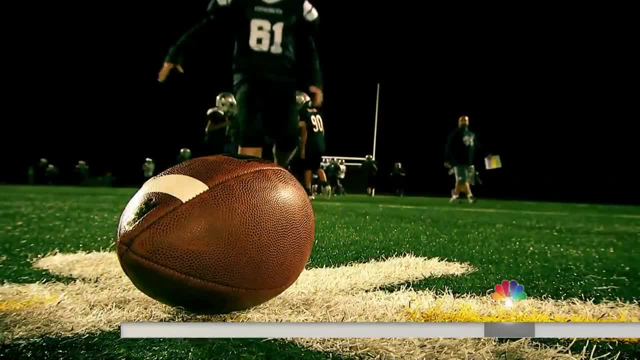 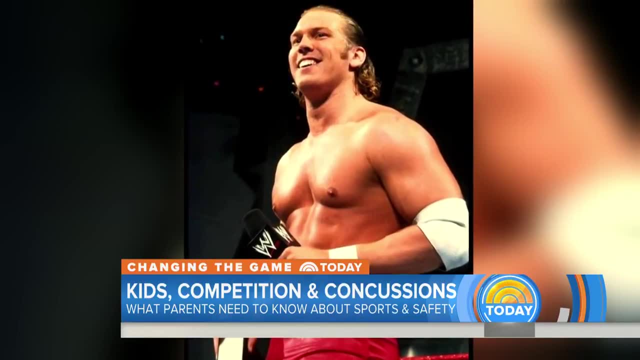 But it's not just for kids with head injuries. The become involved with U S society at 18 every years. In recent years, the number of diagnosed concussions has shot up, Suggesting we're getting better at identifying the symptoms. But is it enough? 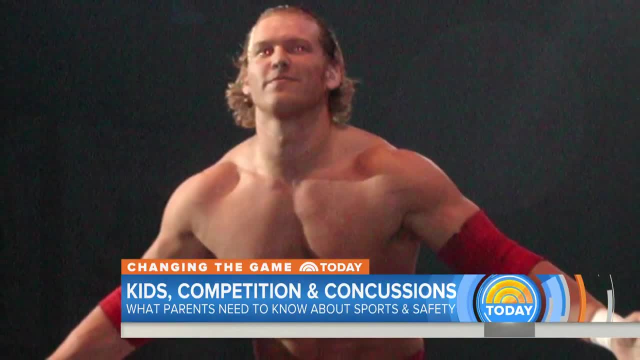 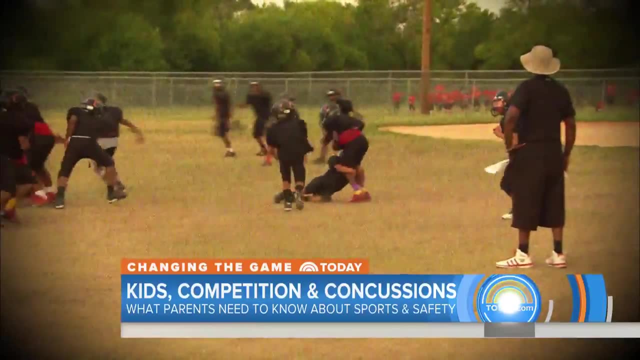 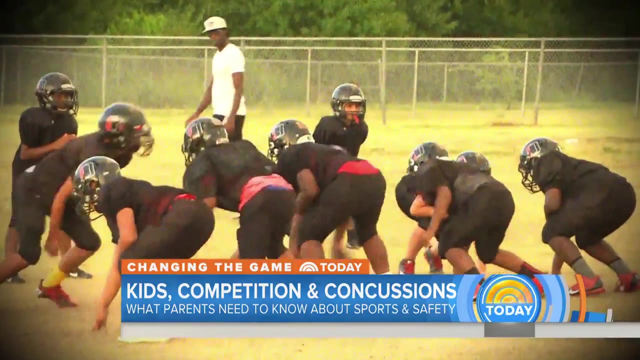 The idea that we have this concussion issue under control is a myth. Chris novelz's, a former pro wrestler who has battled multiple head injuries, co founds it that concussion legacy foundation. We're still not recognizing all the concussions- sub-concussive injury, where you may not even feel it adds up over time. The brain is not meant to. 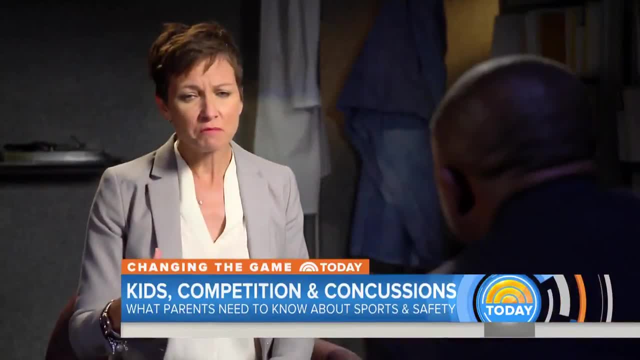 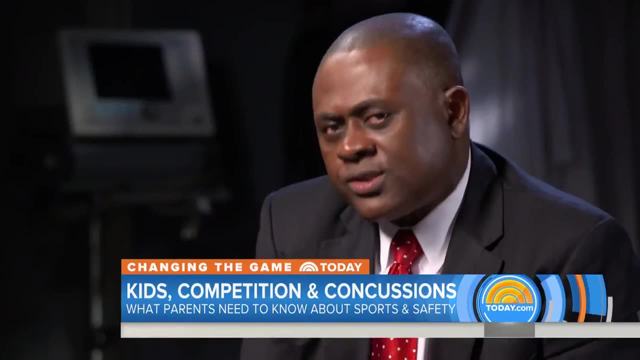 take 500 or 1,000 hits to the head while you're still developing? Do you think parents have a false sense of security that if it's not labeled a concussion then their child is fine? Yes, and I blame we doctors for it. Dr Bennett Omalu, author of Truth Doesn't Have a Side. 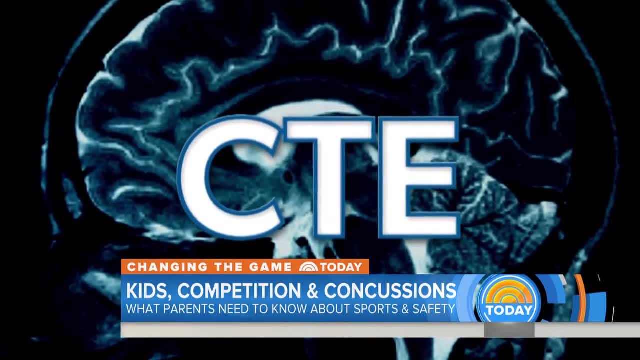 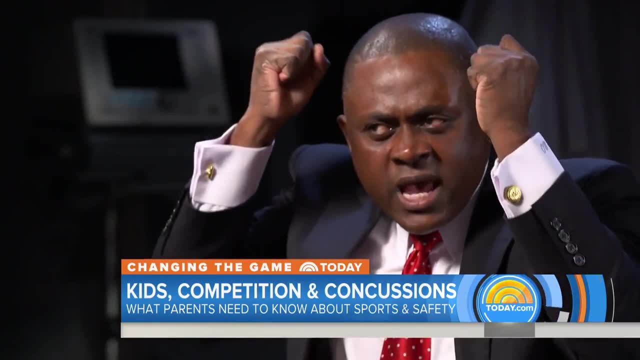 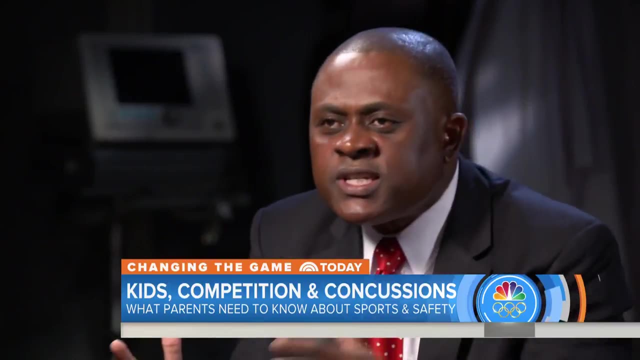 discovered the degenerative brain disease known as CTE. The forensic pathologist who was portrayed by Will Smith in the movie Concussion stirs up controversy If you place a helmet on the head of a child and take that child to a field and he suffers repeated blows to his head over time. 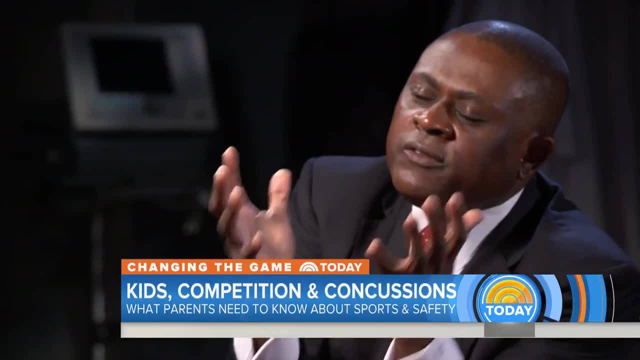 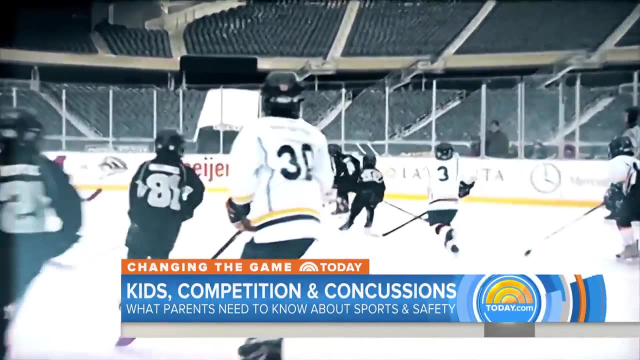 that child suffers brain damage. If that is not the definition of child abuse, what is it? Omalu says children should not play football, ice hockey, rugby, lacrosse and soccer, at least not until high school. But what are we supposed to do? 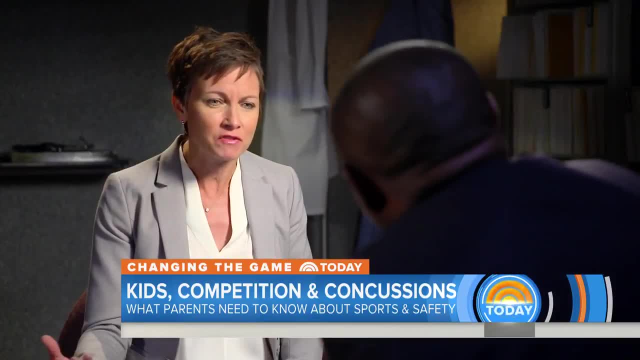 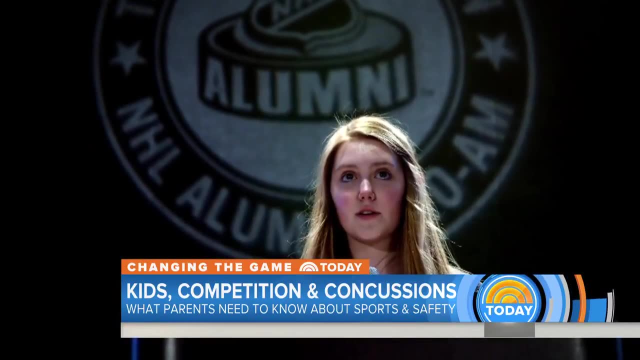 right, We're supposed to wrap our kids up in mattresses and keep them in their bedrooms for their entire lives. There has to be something that we can do. What should kids play? The healthy sports, the non-contact sports. But Esther Lovett, a high school senior who lives outside Boston. 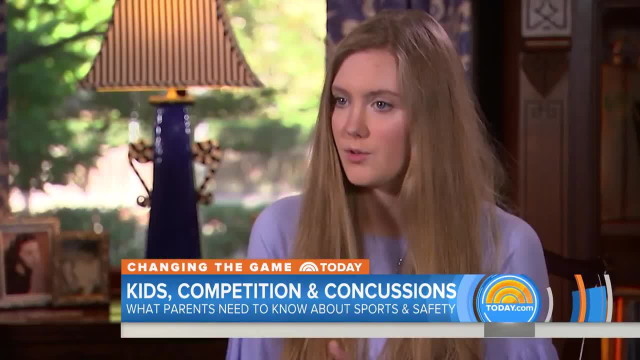 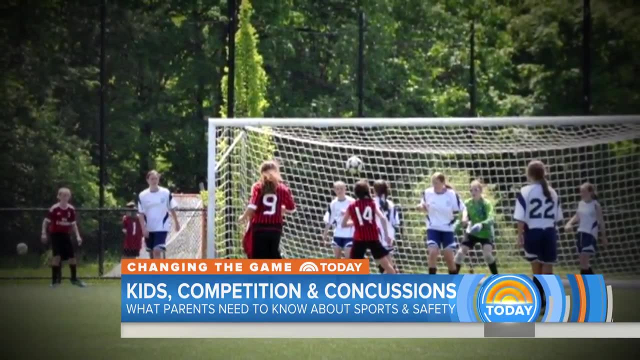 wouldn't trade a day of playing a sport she loves. I'm so thankful for all of my time that I spent playing soccer. Lovett will never play again. after a concussion she suffered in the eighth grade. A girl took a shot on goal and nailed me kind of in the back of the head. 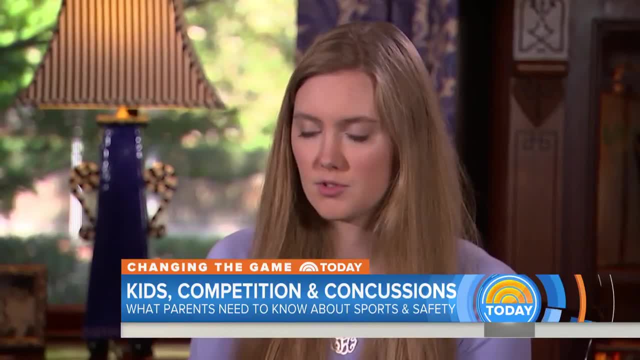 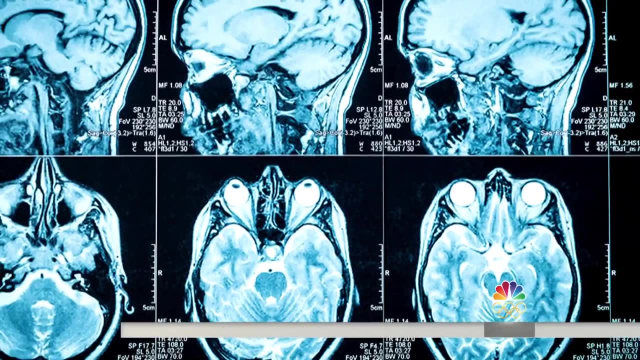 With the ball. With the ball, yeah, And I was really nauseous, pretty dizzy, couldn't really see very well. I played the rest of the game, I just didn't really know any better. The concussion led to a condition that gets. 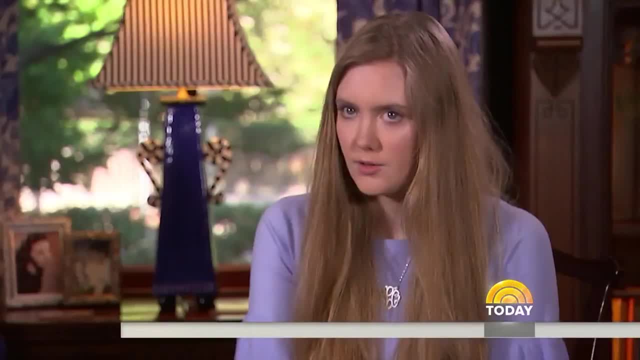 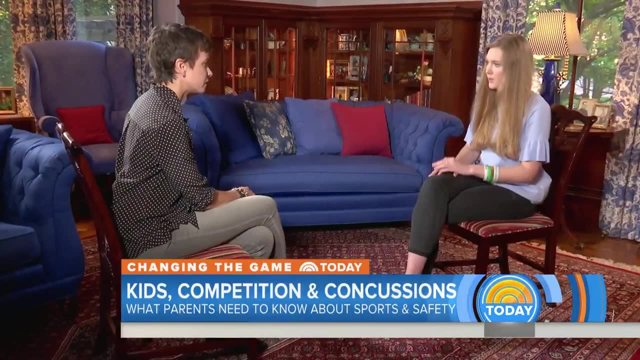 very little public attention. post-concussion syndrome. I don't think I sat through an entire class the rest of that year Describe to me what it felt like, Just like awful headaches Seeing the board. it was just like kind of blurring in and out. 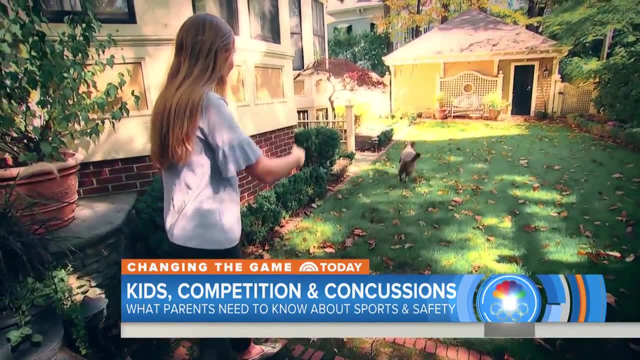 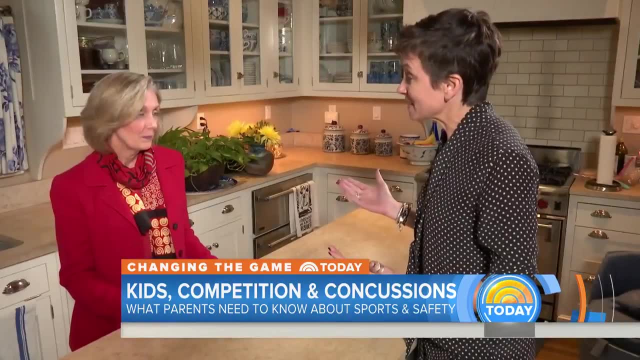 The severe symptoms lasted months. Compounding the problem, Esther banged her head again on the stairs. Years later, she is still suffering from concussion. She is still suffering from daily headaches. Did you ever have any idea that that was in jeopardy Playing that game? 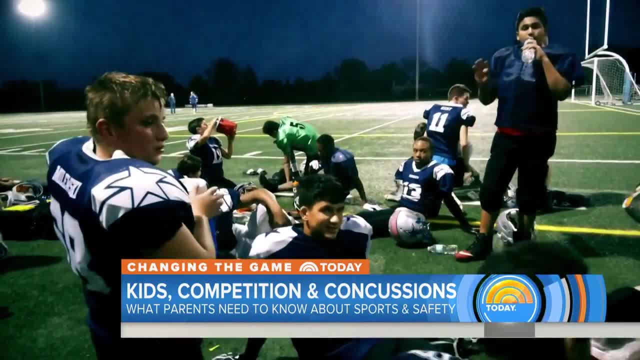 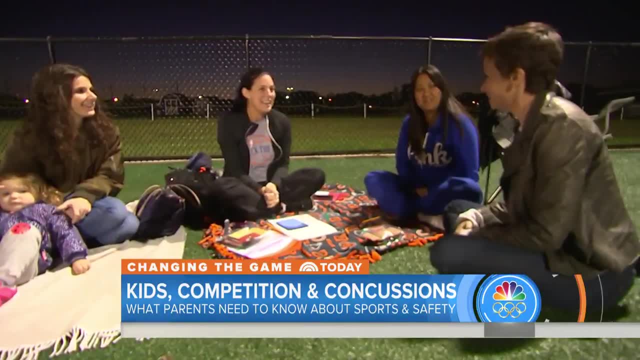 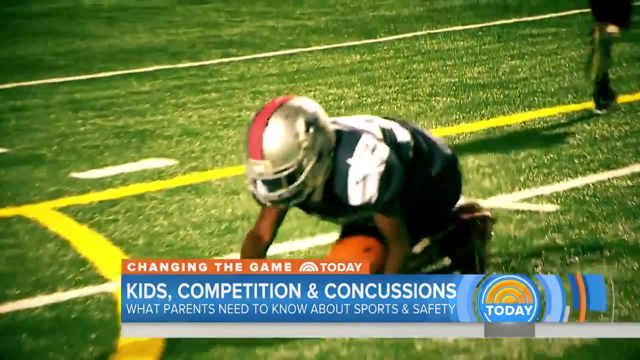 Never, Never would have occurred to us In Addison. this group of football moms is out here every night, every practice. That is some serious dedication. It's fun to watch. They told me they worry about the hits but feel the benefits of playing the sport outweigh the risks.